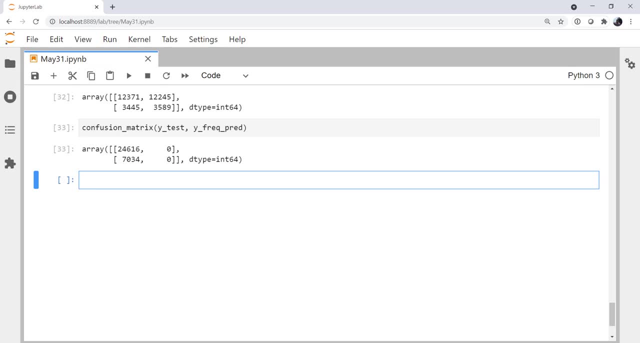 We can use certain scores to accomplish that goal. So we're going to go a little bit further this week and we're going to look at some. We're going to go ahead and get a confusion matrix as a variable here. I'm going to call: 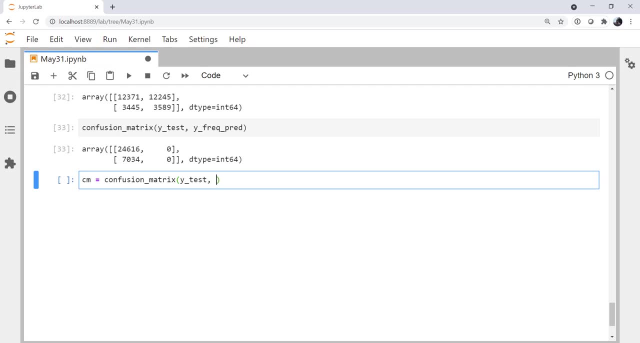 it cm and it's going to be on our y-test and y-predicted data. This is using the notebook that we've been working on for the last couple weeks. This is a k-nearest neighbors. The first thing that we're going to talk about is accuracy, and we've already talked about 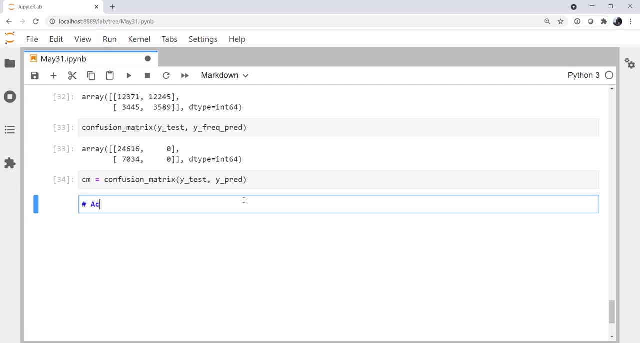 accuracy some in that we've used it but we never have really defined it. What is accuracy? Accuracy is the true positives plus the true negatives, so how much did we get right divided by everything that is in the data set? True positives? 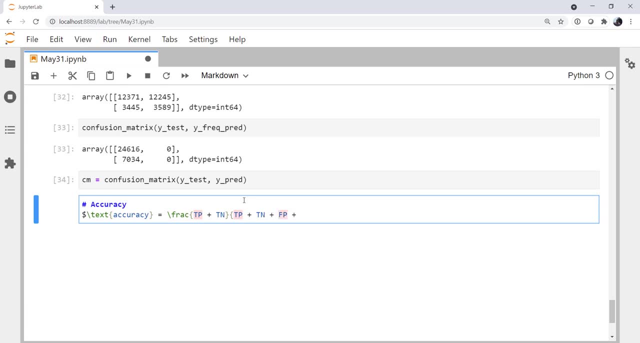 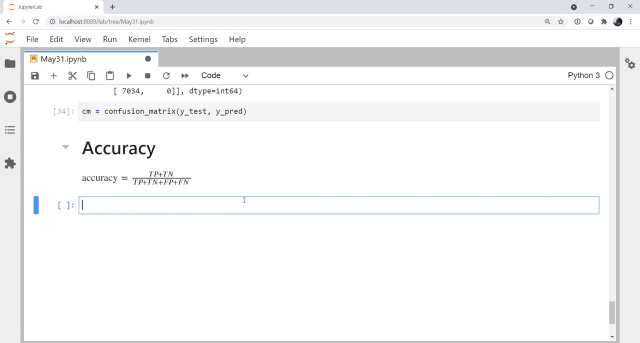 True, negatives, False positives And false negatives: There's our formula for accuracy. So how many predictions out of the whole were correct is what this tells us. We've already talked about how this can sometimes mislead us, especially on things like imbalanced. 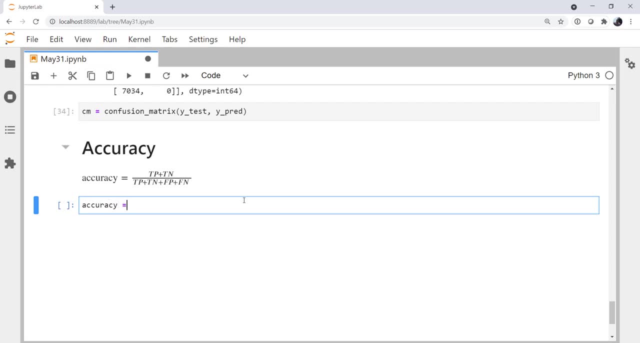 data sets. But let's go ahead and calculate accuracy, longhand, Mark, confusion, matrix. We're going to take the x, We're going to take the element 0, 0.. The element 1, 1.. So we're taking that diagonal. 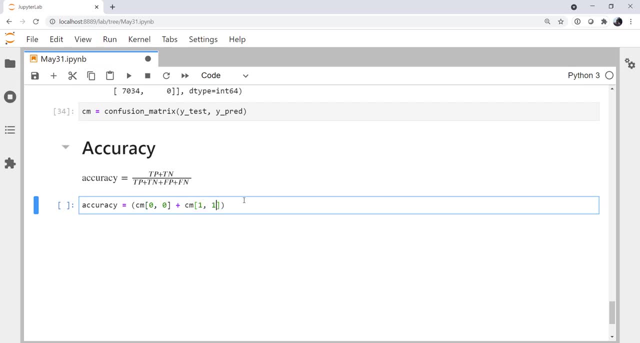 And then we're going to divide that by every element of the matrix, summed So 0, 0.. 0, 1.. 1, 0.. And 1, 1.. And we'll print that out. So 1, 0.. 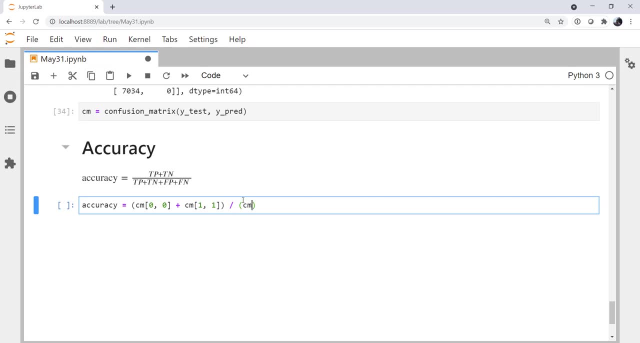 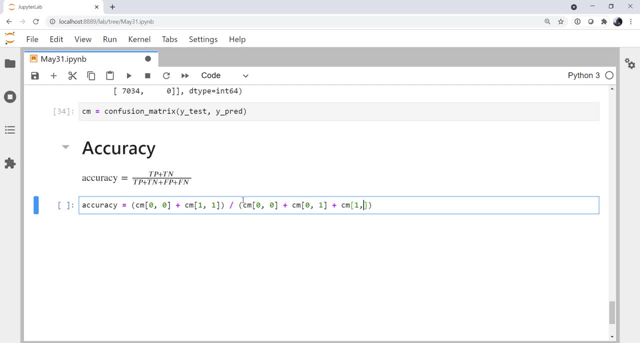 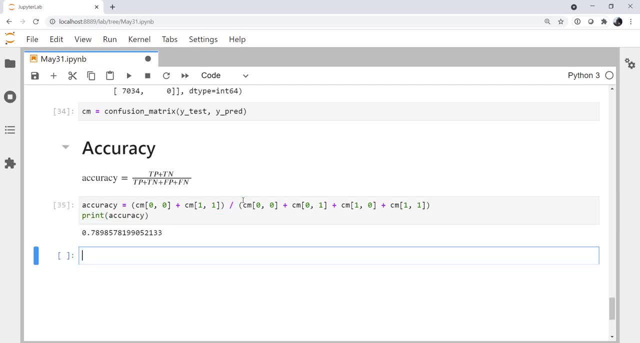 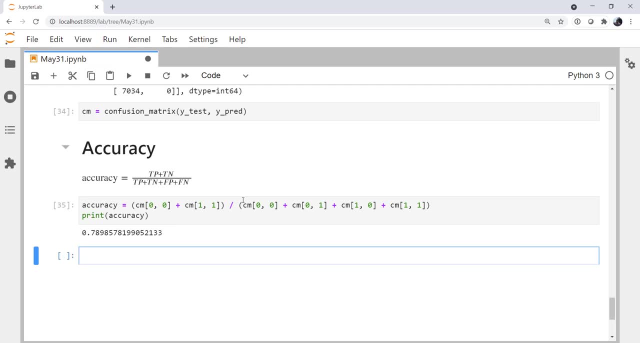 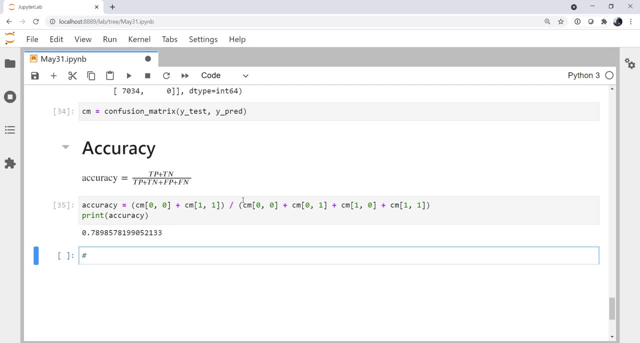 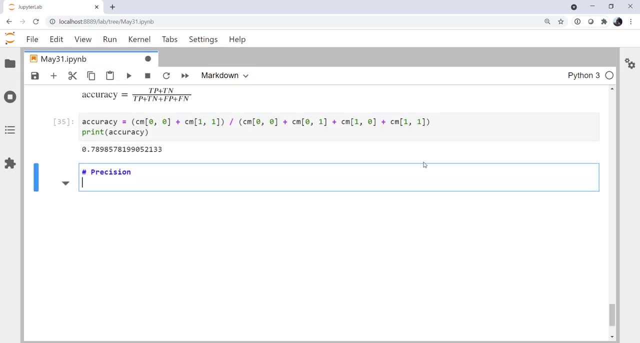 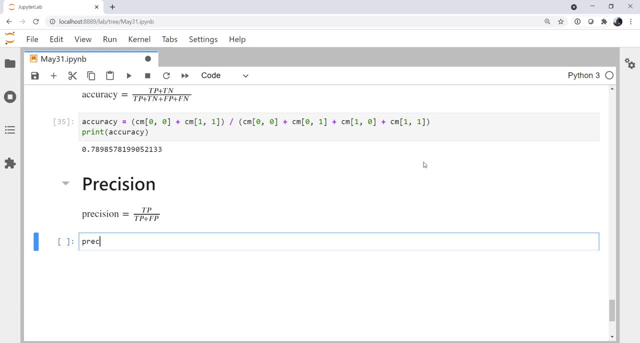 there's our formula. let's go ahead and calculate it. so the numerator is element 1: 1 of our confusion matrix. the denominator is element 0: 1 plus element 1: 1, and we get a precision of 53.5. so when would you use? 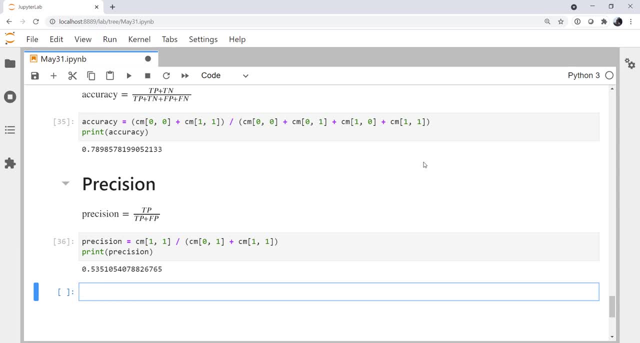 precision. well, like I said, it says how many positives are actually positive. so we're wanting to limit the number of false positives. if we're optimizing for precision- and you may also see this in some literature, referred to as the positive predictive value or PPV- it's important to understand the strengths and weaknesses. 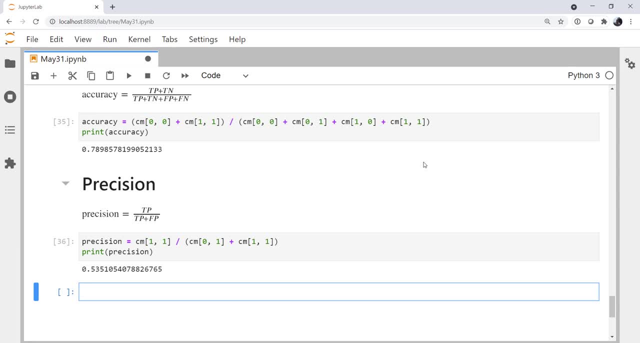 of all of these that we're going to go through, because they can be used to sell you an algorithm, because you can make any one of these numbers look pretty good or even perfect, as we'll see. but you really have to take into account the performance overall of the number of false positives and the number of positive. 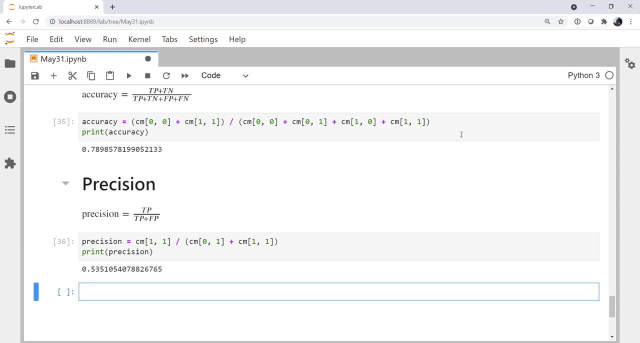 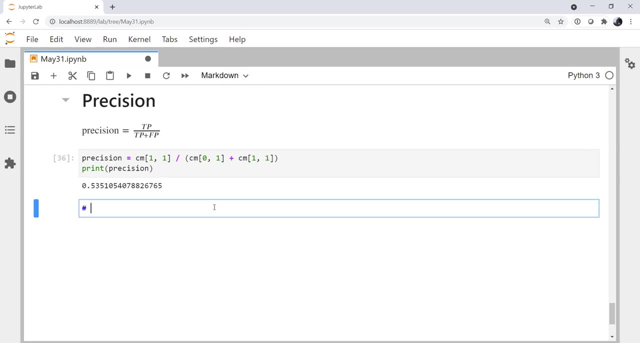 and what your use case is. all right. so what about recall? accuracy and precision we're somewhat familiar with from our normal scientific training, but recall is most likely new. the formula for recall is in the numerator of our fraction true positives and the denominator true positives plus false negatives. 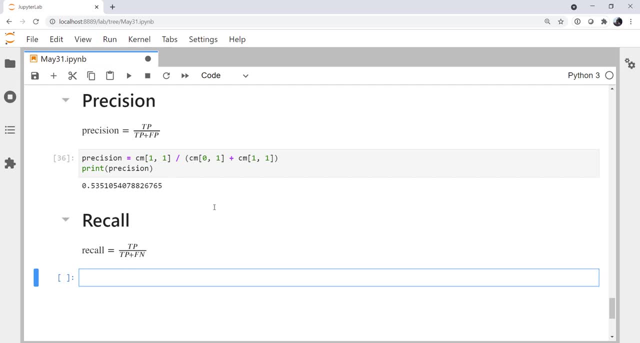 so recall measures, how many positive samples are captured by the positive predictions. so this means our goal is to avoid false negatives. we don't want to miss anything. we're okay with some false positives. you see, false positives are nowhere in this equation. in fact, precision and recall are somewhat. 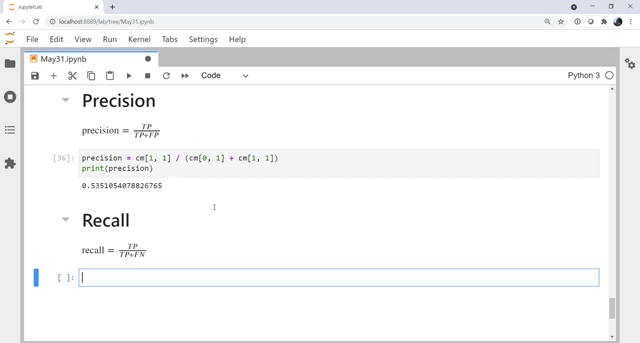 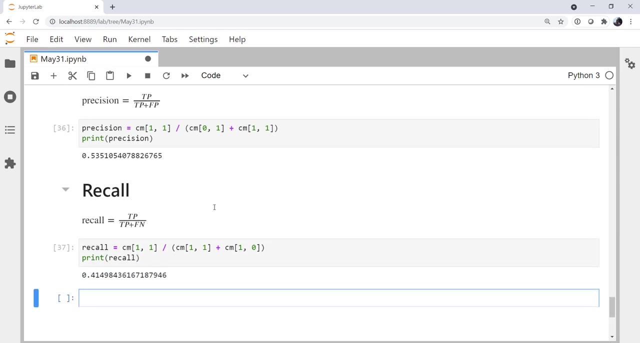 opposed to each other. you can't really have both. you can optimize for one or the other and it's what you're looking for. goal is: let's calculate recall. element 1: 1 is our true positives. we divide that by the sum of element 1: 1 and 1: 0- that bottom row- and for our recall we get 41.5. not a fantastic score. and we're, remember, we're going to avoid false negatives here, so we're not doing very good at that, which means in our case, the rain situation is what we're predicting is positive. when I talked about being able to sort of a game seeing these metrics, remember if you predicted all positives, you would have perfect recall, because we are not penalizing in any way for false positives, we're only penalizing for false positives. 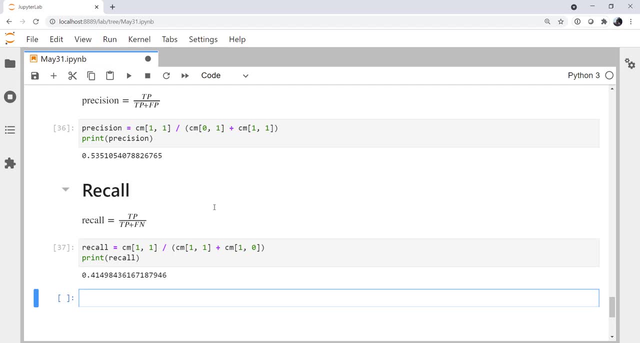 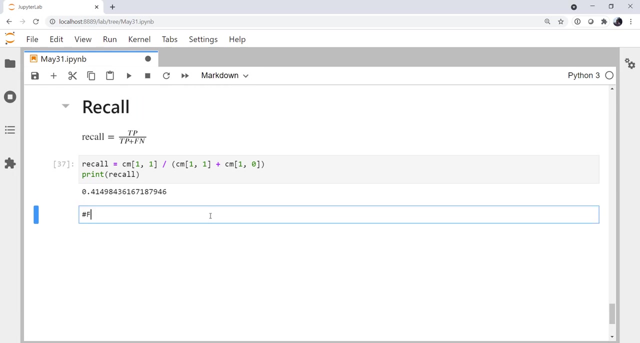 negatives here so that one can look very good depending on the situation. so precision and recall have this trade-off and you have to balance them. one way we can do that is by looking at the f1 score. there are various F scores. f1 is probably the most common f1 score. the formula for the f1 score, f sub 1, is the: 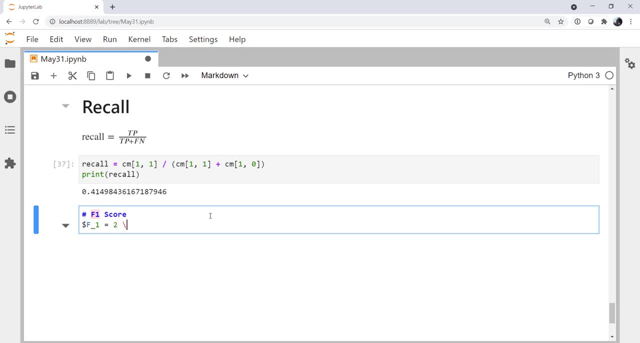 population and that's going to depend on our formula, what we're going to call the F-1 score. that, just in general, it becomes a question we need to understand- does a good. this is what impf that basically is. so this is what we're going we do, we just. 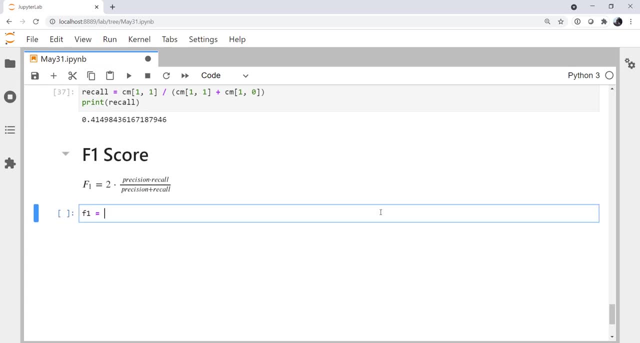 basically that is what we play: one point, one point. calculate it. Remember to use tab completion and save yourself some typing and typos. Our F1 score is 46.7.. F1 scores do a really good job, helping you not be fooled by imbalanced 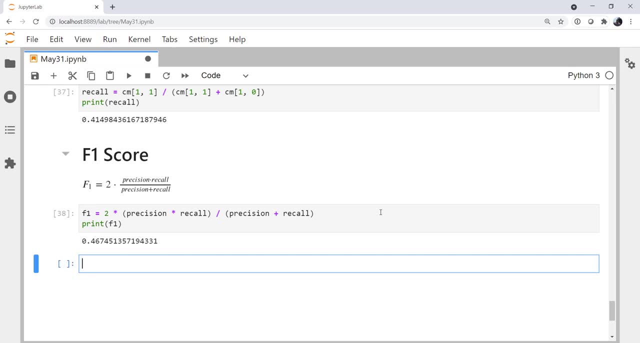 binary classification, which is exactly what we have here. We have binary classification- rain or no- and it's very imbalanced because most of the data set is the no rain case. So now that I've showed you how to calculate all these and we understand where they come, 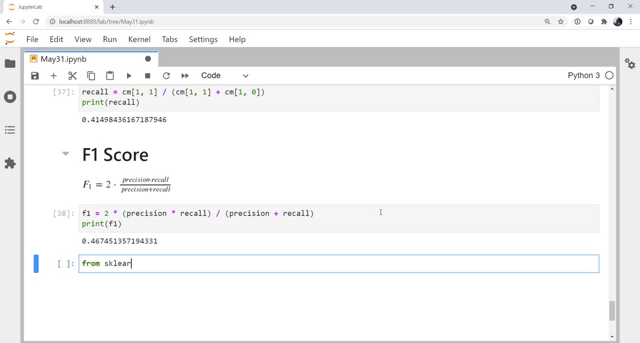 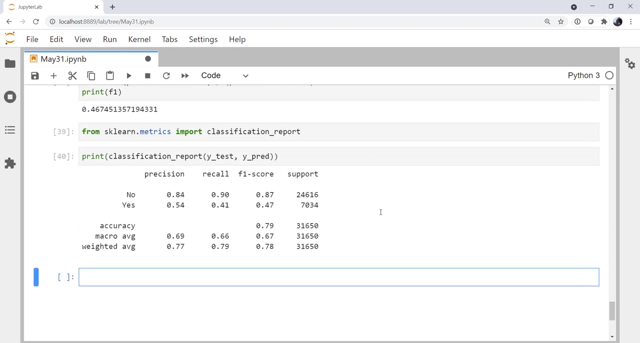 from and what they are. we're going to look at. in the metrics module of scikit-learn, this function called classification report. If we print the output of the classification report- our ytest data, and say our ypred data from the k-nearest neighbors, you see that it actually calculates all of these for us. 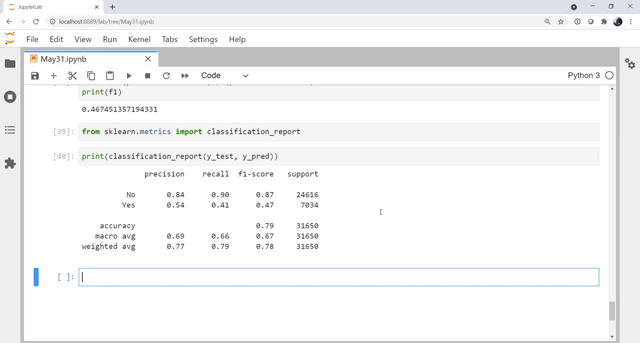 So we've got precision recall F1 score and how many data points are supporting that, And you can also see we have no and yes are two cases. Is it going to rain? And it shows each one of those as if they were the positive. So for yes, which is the problem that we've 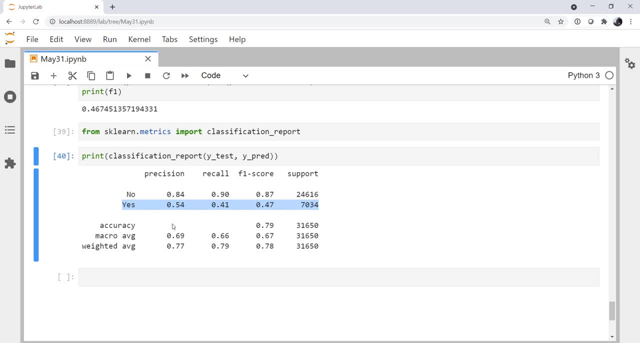 solved so far. we get numbers that match what we've calculated by hand above. But for no, if we say no, rain is the positive case. that's what we care to predict. we can see the scores are much higher Again just because, well, there's not as much rain If we look down. 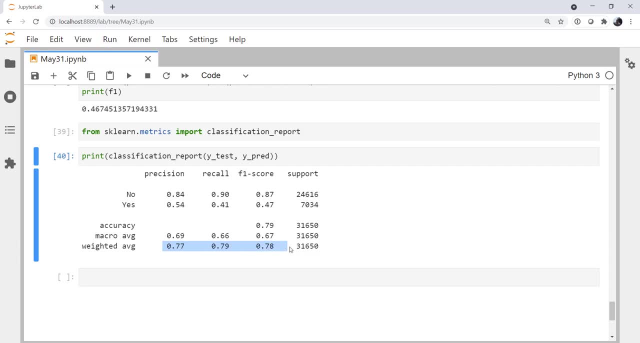 here. at these averages, though, where we take the weighted average especially. based on this, we can really get an idea of how do we do, And it's not stellar. yet We haven't really optimized our hyperparameters, We haven't tested other methods, We haven't looked at